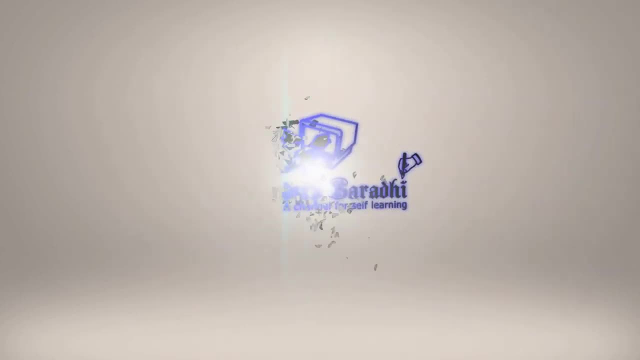 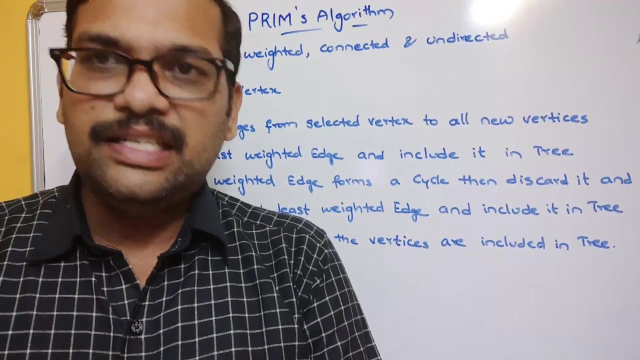 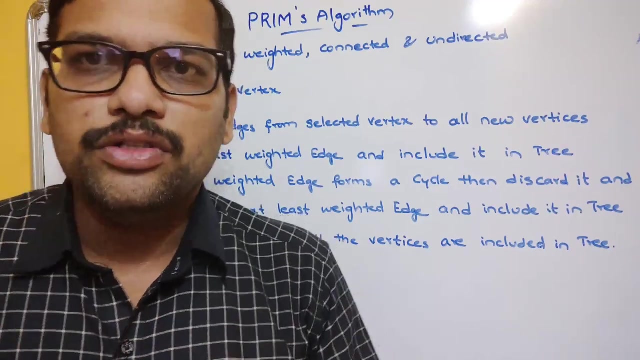 Hello friends, welcome back to our channel. So in the previous session we have discussed about what is a spanning tree and what is a minimum cost spanning tree. So in today's session we'll discuss about how to find that minimum cost spanning tree. So here there are two approaches. 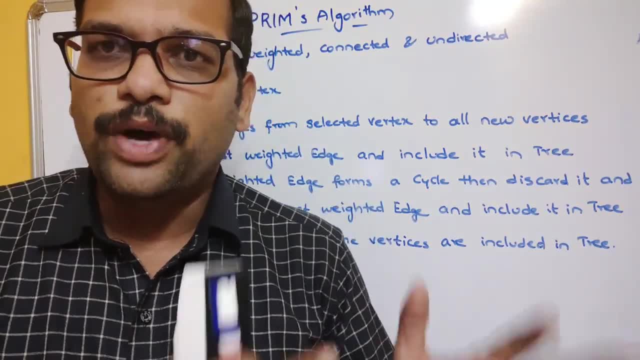 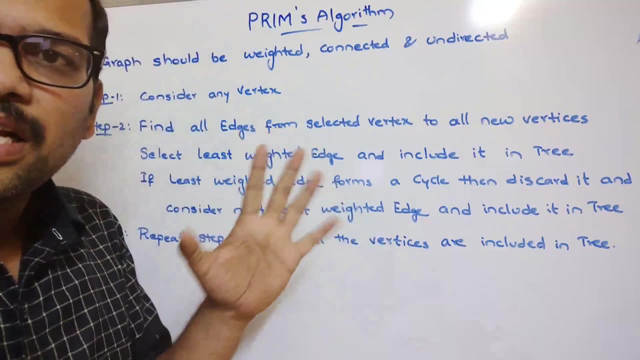 to find the minimum cost spanning tree from a graph. So that is one is a Prim's algorithm, another one is a Kruskal's algorithm. So in today's session we'll discuss about the Prim's algorithm. So before applying the Prim's algorithm on the graph, make sure that the graph should be. 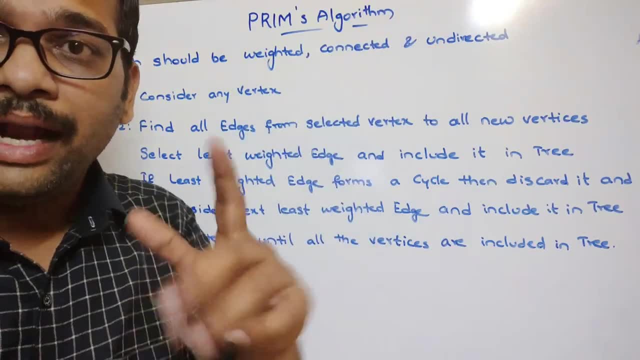 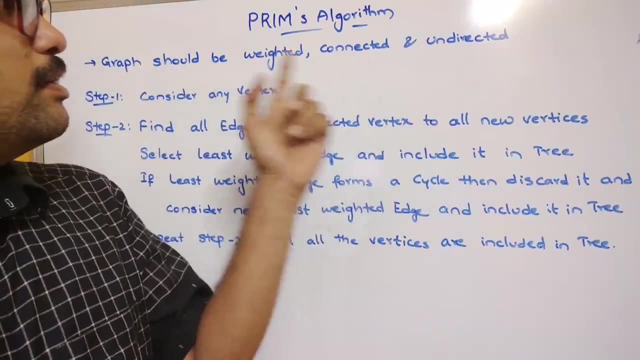 weighted, connected and undirected. So unless the graph is weighted, connected or undirected, so we can't apply the Prim's algorithm. So make sure the first point before applying the Prim's algorithm: So the graph should be weighted, connected and undirected. And coming to the 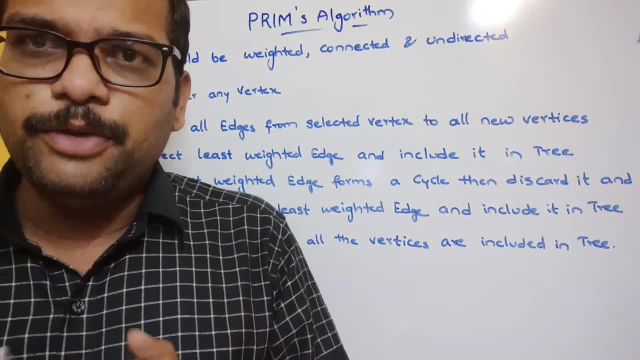 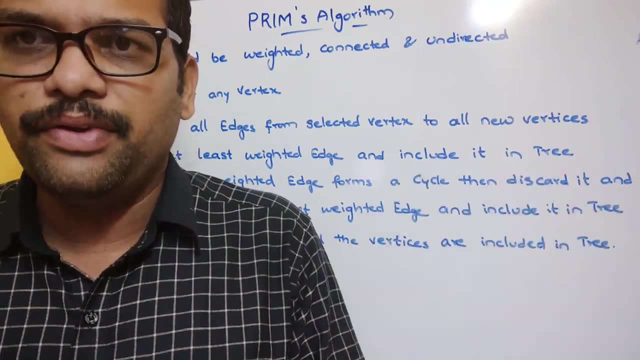 steps. So first we need to consider any vertex, because so we know the spanning tree definition. Spanning tree is a subgraph from the graph, without any cycles, consisting of all the vertices of a graph. So consider any vertex of the graph And the second step, find all the edges from the 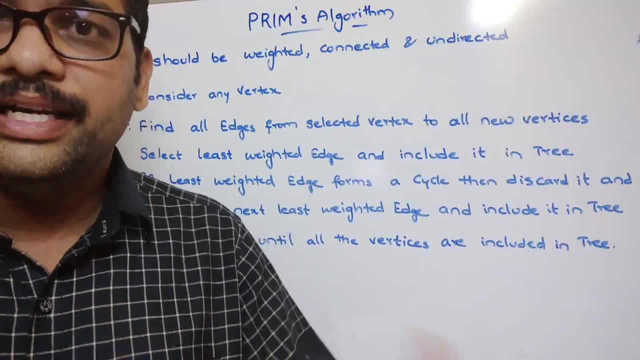 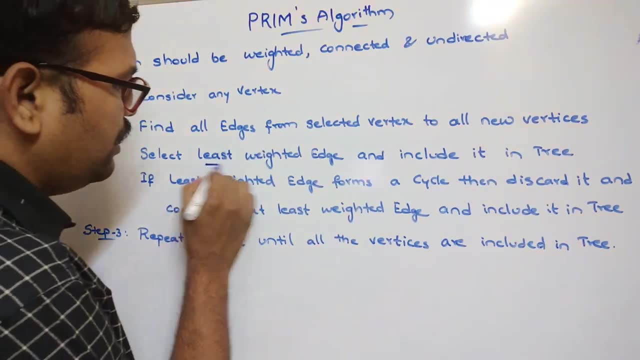 selected vertex to all the new vertices. So find all the edges. So among all the edges you need to select the least weighted edge. So among all the edges, we need to find the least weighted edge and include it in a tree. So we need to construct a tree for that selected vertex and give in the 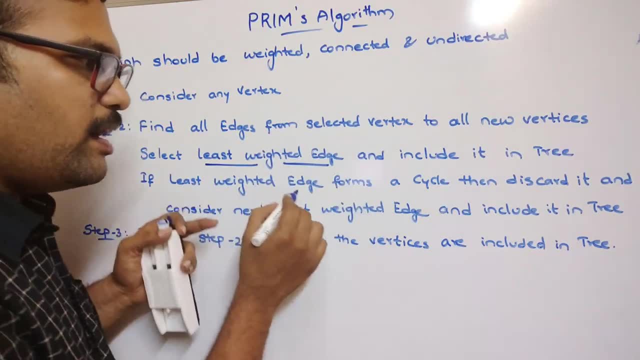 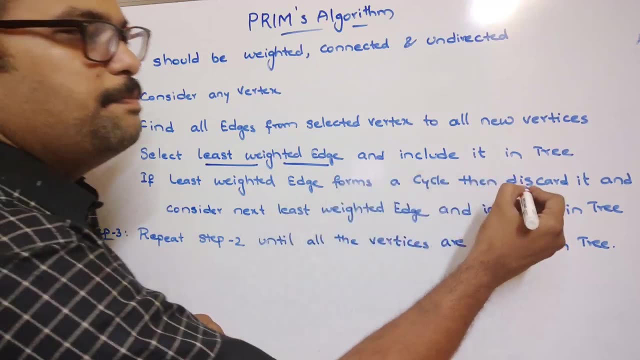 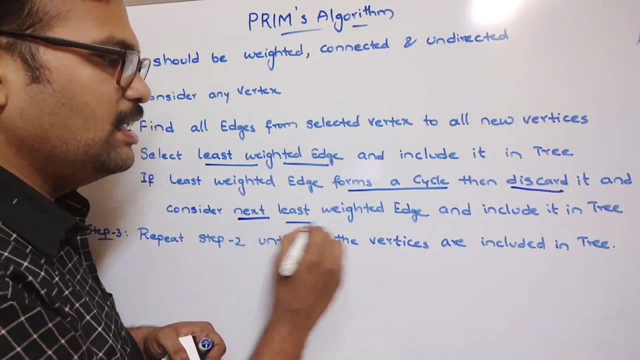 least weighted edge And if the least weighted edge forms a cycle. So if you include this least weighted edge into a tree and if it forms a cycle, then simply discard. So it forms a cycle, then simply discard that one and consider the next least weighted edge. So once you find the 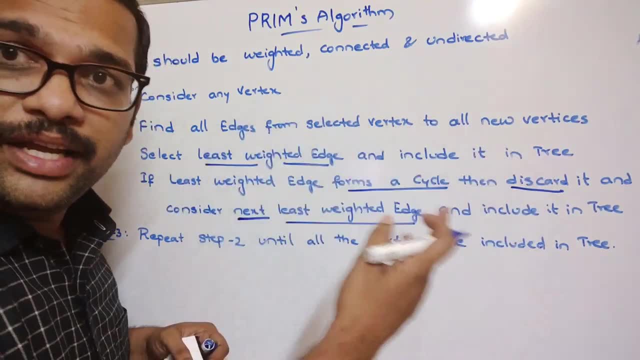 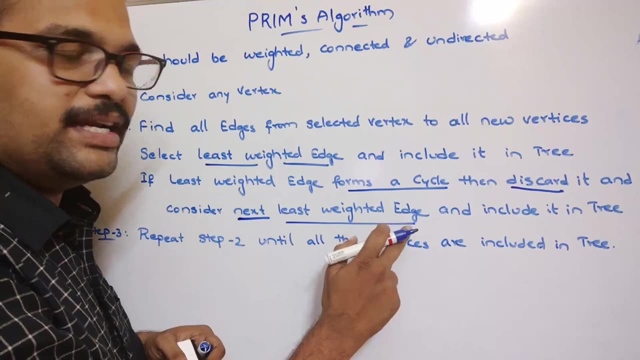 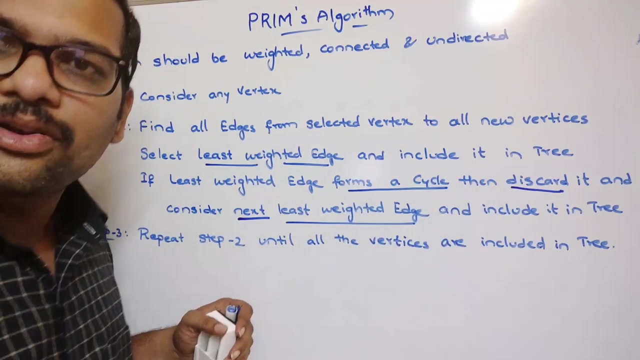 least weighted edge, you have to include it in a tree. So, after including it in a tree, you need to. if it forms a cycle, simply discard that one and consider the next least weighted edge and include it in tree. And the third step: repeat the same step two until all the vertices are included in a 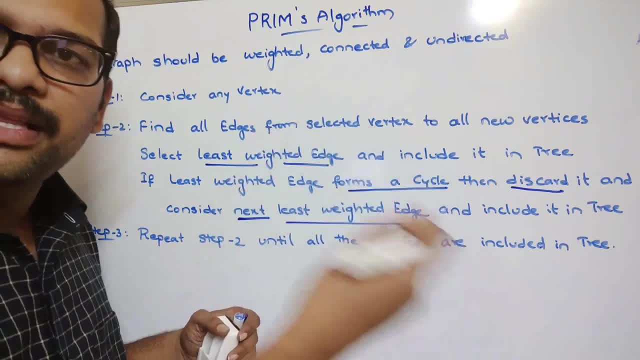 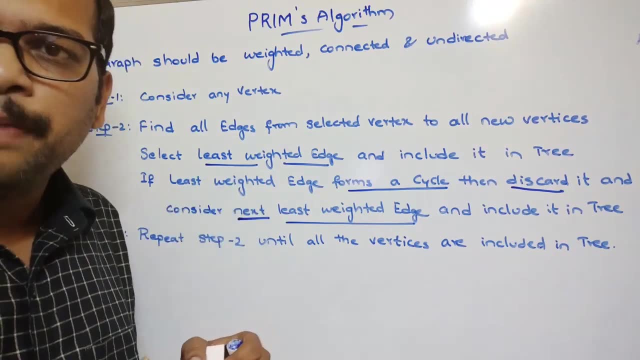 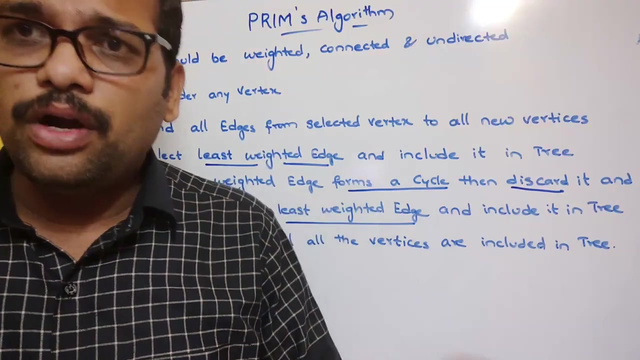 tree. So once all the vertices are included automatically, that will be the minimum cost spanning tree. So this is how we need to find the minimum cost spanning tree with a PRINCE algorithm. In our previous video on data structures and algorithms, many of them were asking about 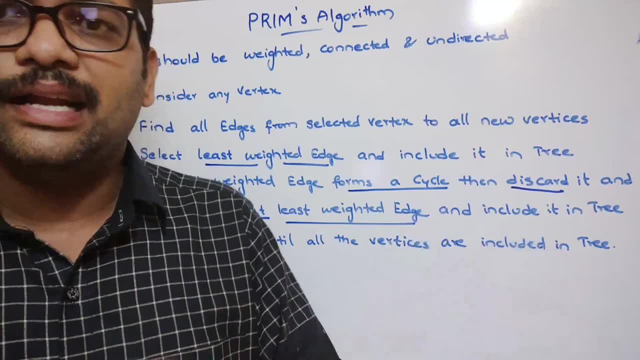 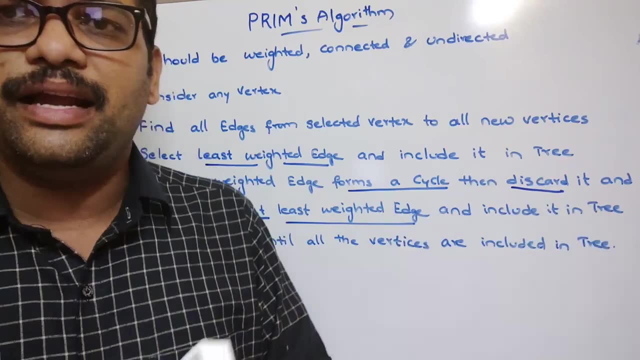 upload more number of videos on the data structures and algorithms. So, in this regard, I want to tell you that Anacademy has started a course regarding the data structures and algorithms, partnering with the Lovebubble. So if anyone wants to get a job in data analytics or 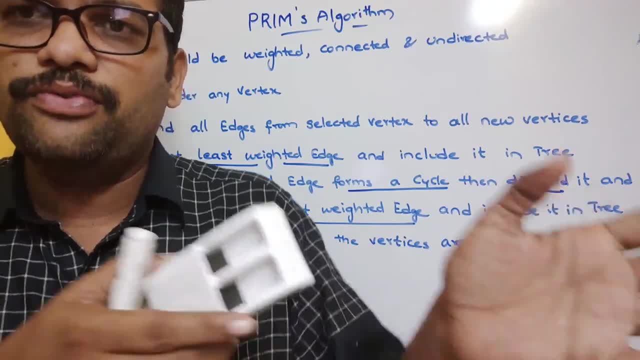 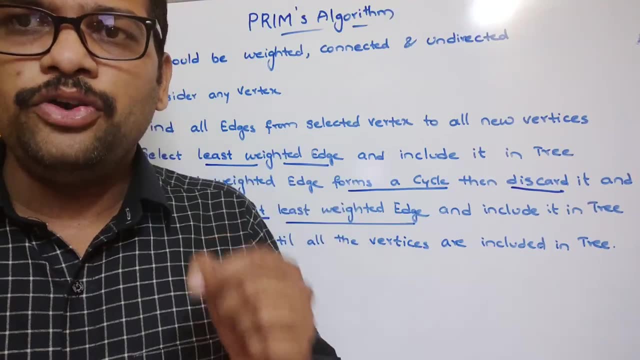 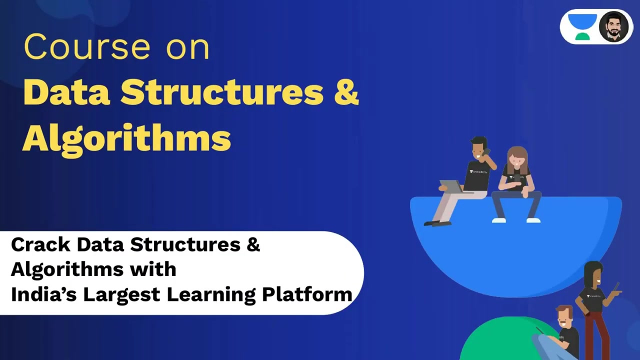 in a topmost tech giant companies like Microsoft or Amazon, etc. etc. you need an in-depth knowledge on data structures and algorithms. So enroll yourself in the course given by the Anacademy and crack it, Hello students. If you want to get a good job in a top tech giant companies like 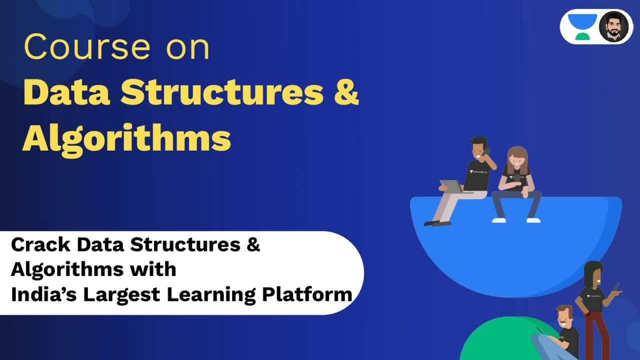 Microsoft, Google or Amazon- that's a product based companies with the highest package. the only one concept you need to concentrate more is on data structures and algorithms. So a normal basic knowledge on data structures and algorithms is not sufficient for those tech giant companies. So if you want to grab a deep knowledge of data structures and algorithms, 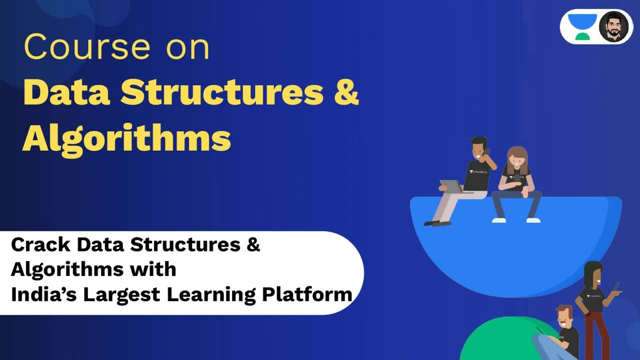 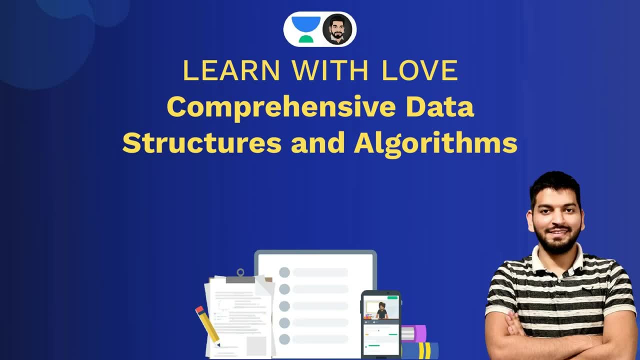 here is a new initiative started by Anacademy, India's largest learning platform, partnering with the Lovebubble, So you can learn with the Lovebubble all about a comprehensive data structures and algorithms. Lovebubble is a software engineer and a YouTuber He worked with 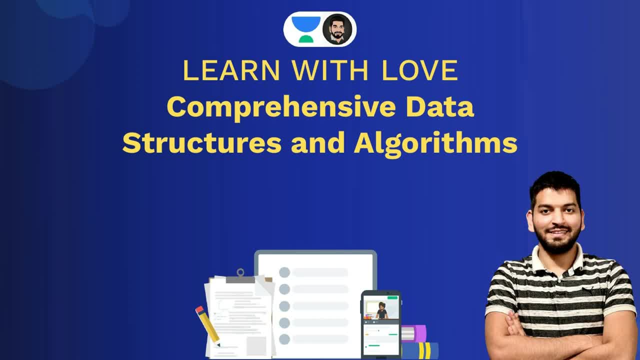 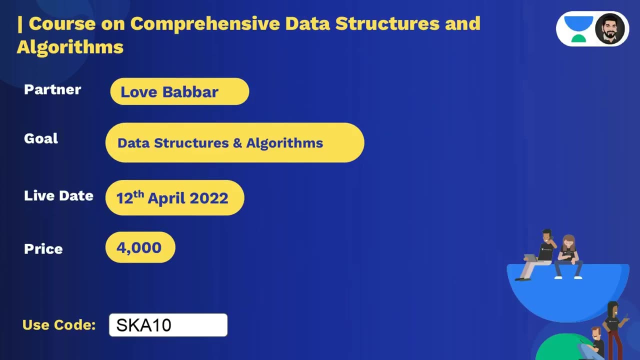 some of the world's most well-known product firms, including Amazon and Microsoft. His software engineering abilities are well known And he also works as a coding tutor for college students and also have mentored over five lakh students till date. Students Anacademy is launching. 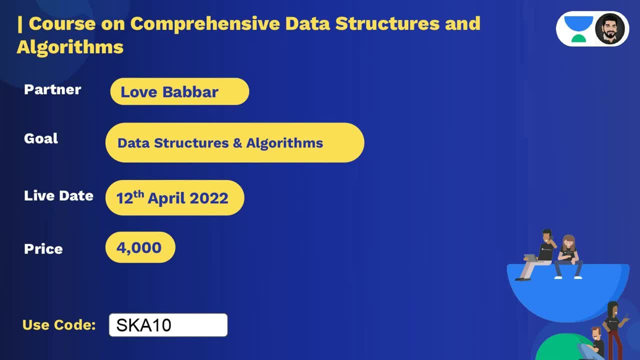 this course on 12th April 2022. And the price of the course is a minimal of 4000 rupees, So there is an early bird discount going on in this Anacademy link Link is mentioned in the description. Check the offer by clicking the link. over and above the early bird offer. 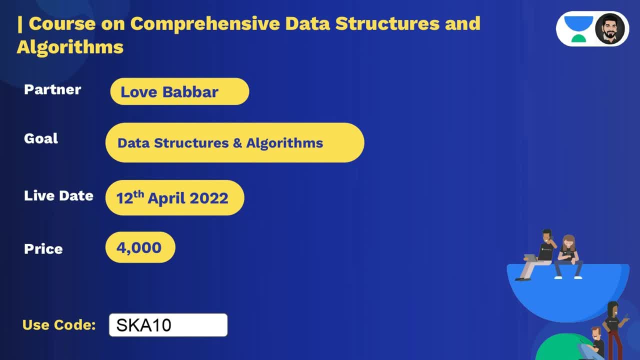 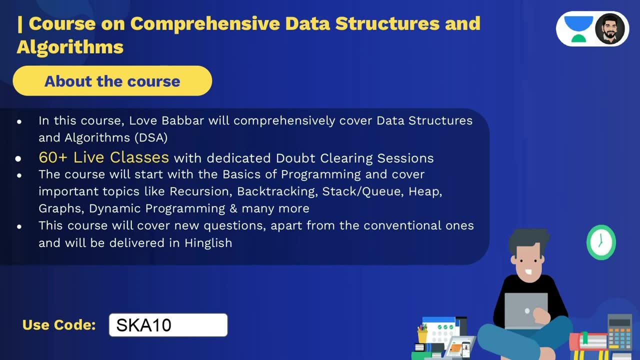 You can avail 10% flat discount by using our referral code SK810.. In this course, Lovebubble will comprehensively cover data structures and algorithms. There will be 60 plus live classes with a dedicated doubt clearing sessions, And the course will start with. 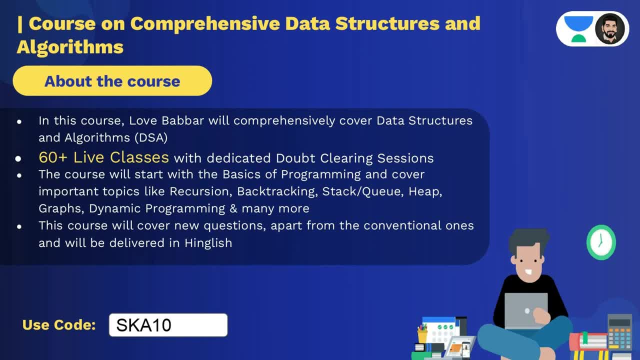 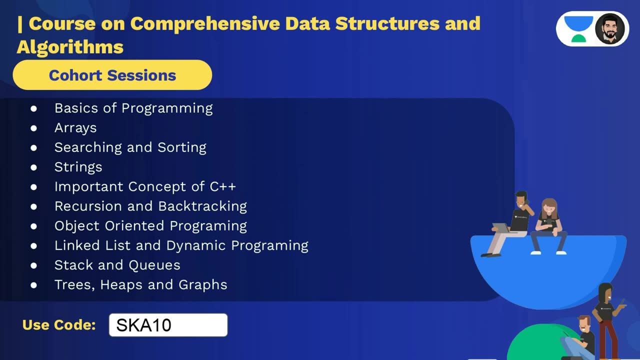 the basics of programming and cover important topics like recursion, backtracking, dynamic programming and many more will be covered. This course will cover a new questions apart from the conventional ones, And there will be 10, three to six chapters and 15 sequential questions, and Delivered in English. 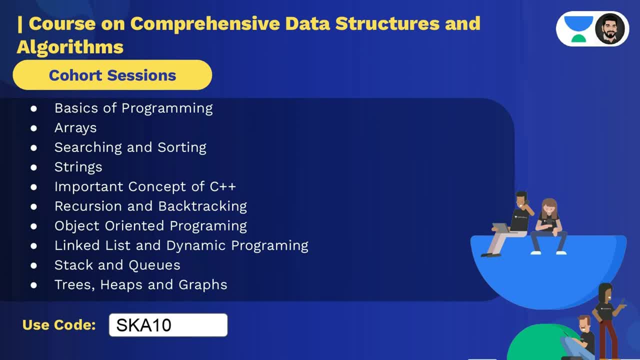 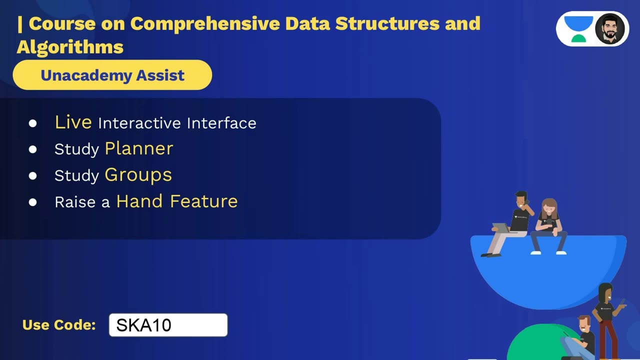 Students in this course. you will be getting a cohort sessions in which Lovebubble will be explaining about basics of programming: arrays, searching and sorting techniques, strings, important concepts of C++, recursion, backtracking, linked list, dynamic programming, etc. And there is also an Anacademy assist feature which consists of live interactive interface. 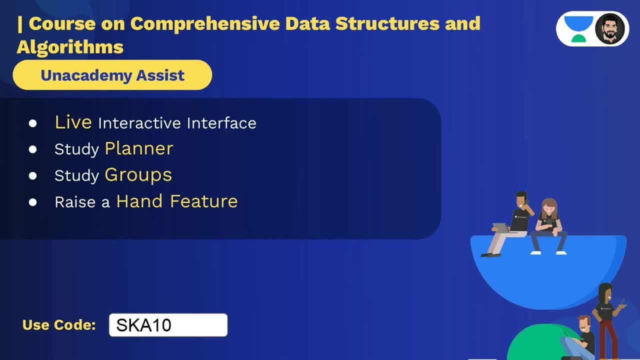 And there will be a study planner And you will also be part of study planner enhancement series. So don't worry, We have lots to learn. Go ahead and explore dasKook groups. so there is a raise a hand feature where you can clear all your doubts during the session. 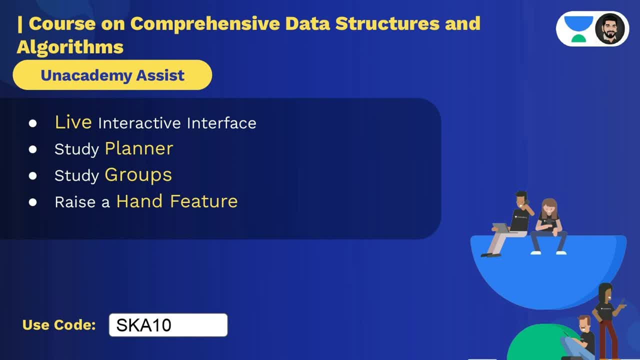 and this is a very good initiative started by an academy. so please do check and avail this course, and the link is available in the description section. you can click on the link and use my referral code, sk810, and avail 10 flat discount. so, my dear students, start your data structure. 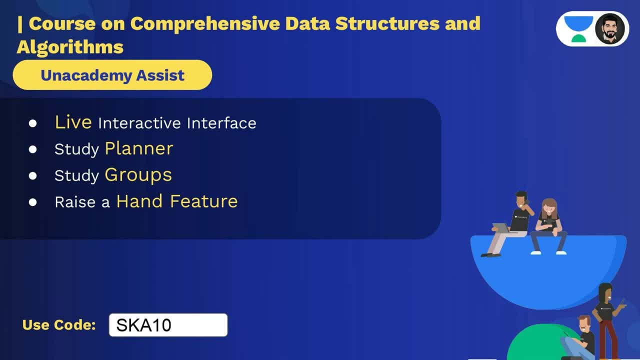 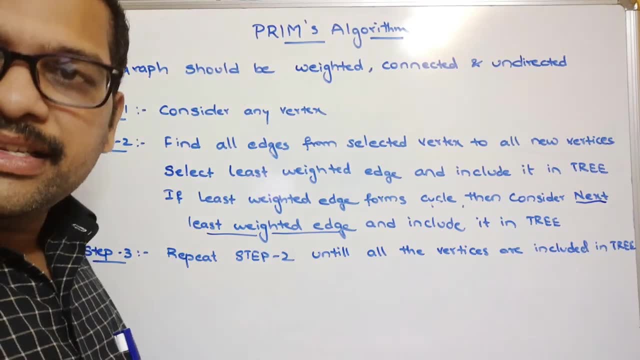 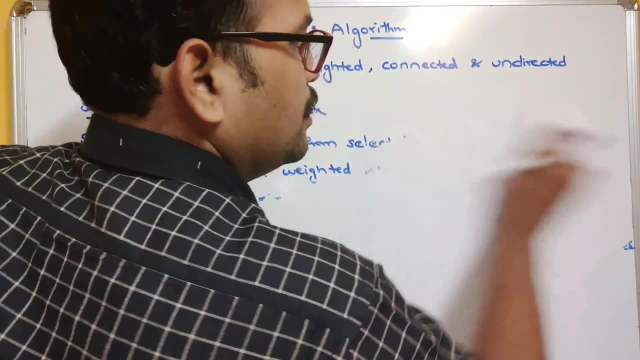 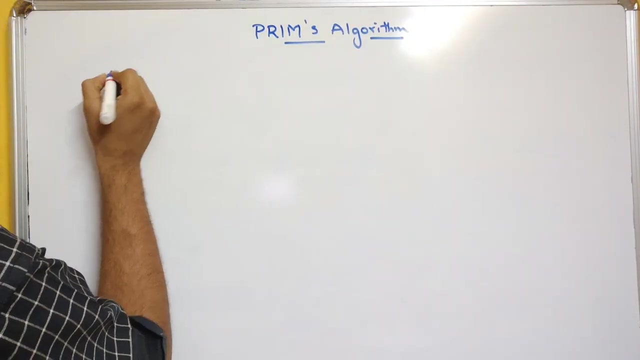 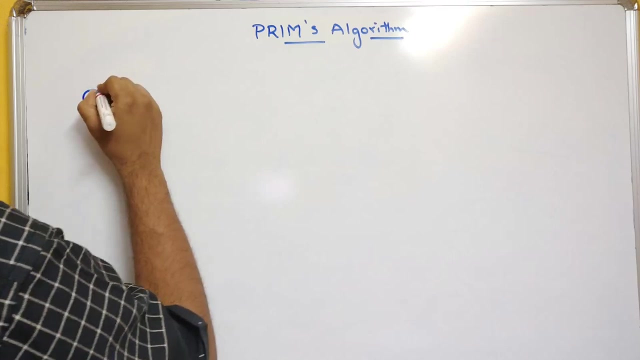 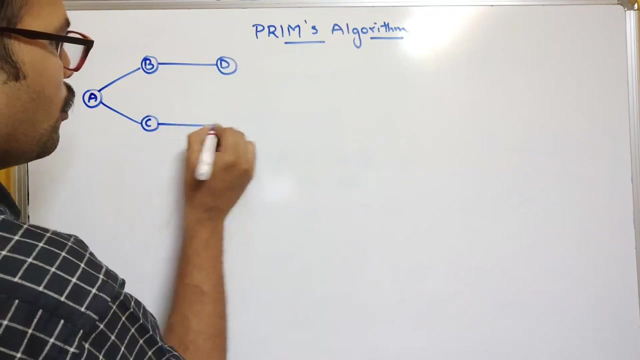 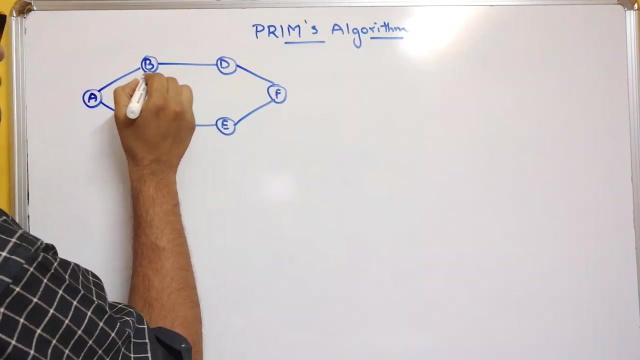 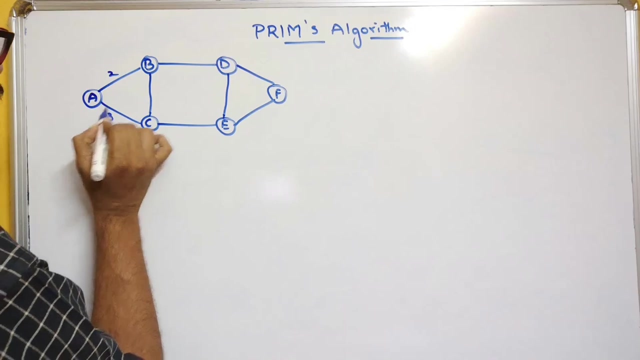 and algorithms learning with an academy, let's crack it. hello friends. so welcome back to our session. so here now we'll see an example and we'll find the minimum cost spanning tree by following all these roots. so let us take an example. so consider one graph. so consider this graph. so let us take some weights. 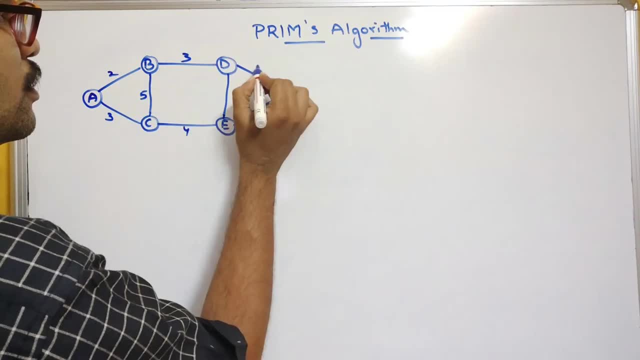 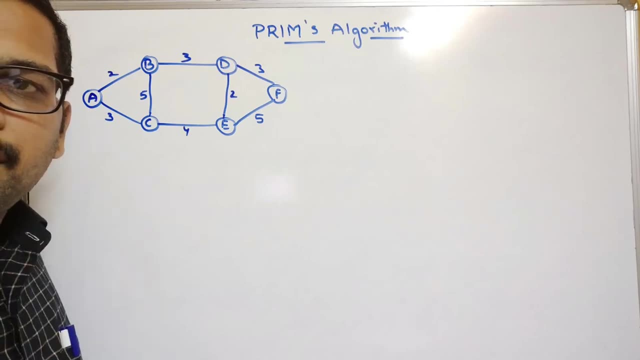 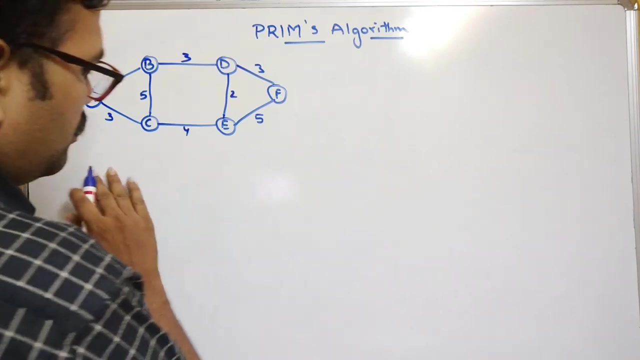 so let's take these weights. okay, this is a graph, consider this graph and we need to find the minimum cost spanning tree for the, the scale. so let's take a graph and we need to find the minimum cost spanning tree for the scale, this particular graph. So what we have to do? First, consider any vertex. So I will. 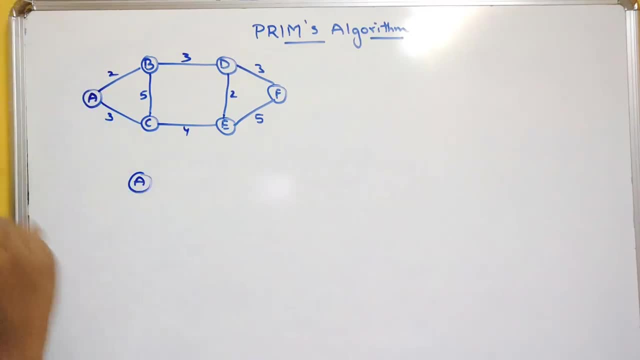 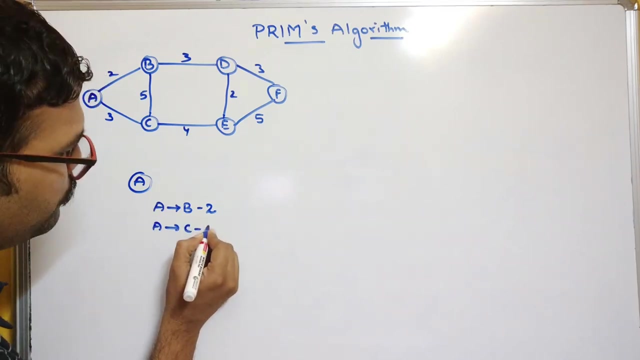 consider A. I will start with A. So this is an A, So I have included this one in the spanning tree. Now consider all the edges from A, So you can see A to B with a cost of 2 and A to C with a cost of 3.. A to B with cost 2, A to C with cost 3.. So we need to. 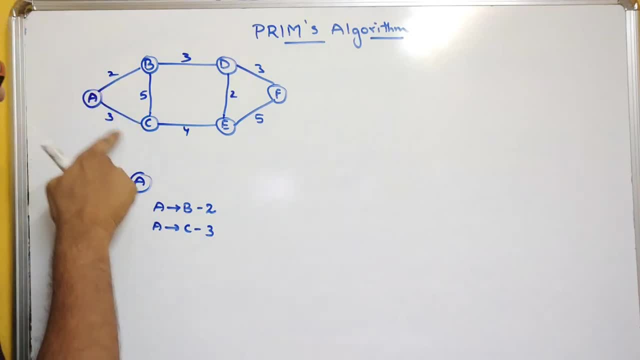 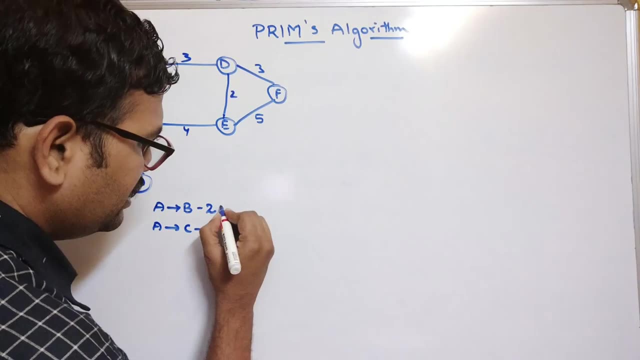 select the least weighted edge, because A is having two edges: One is from A to B, one is A to C, A to B, A to C. So consider the least weight. So this is the least among these two. So we need to add this B to the spanning tree. Now the spanning tree will: 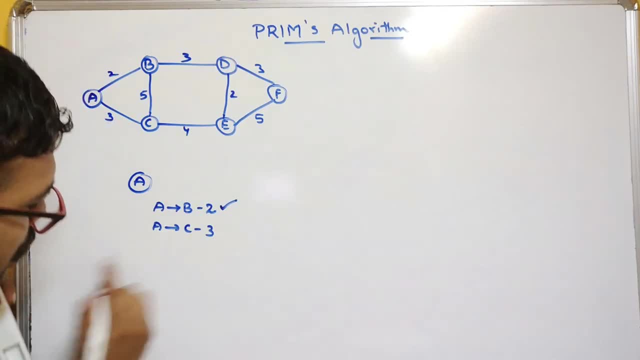 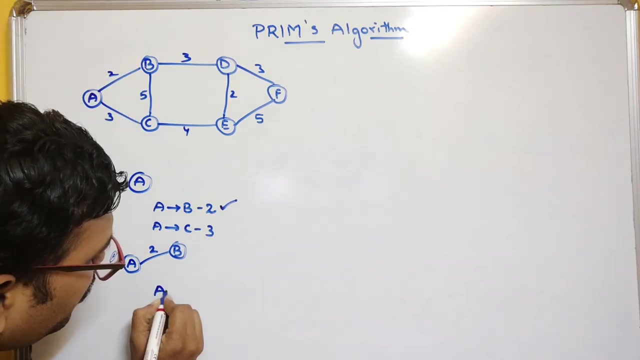 be A, A followed by B, So with a cost 2.. So this is the tree. This is the tree. Now, what is the new vertex here? B. So what is the remaining vertex? Consider this one: A to C, with 3 and. 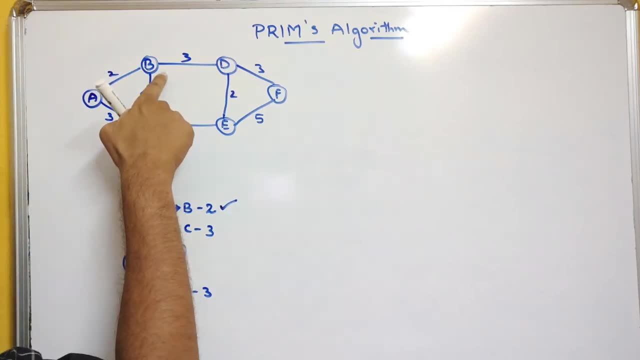 consider the edges from B: right, So from B there is a vertex from B to A, which is already covered. right, Because this is a undirected. okay, This is a undirected, So B to A is covered. 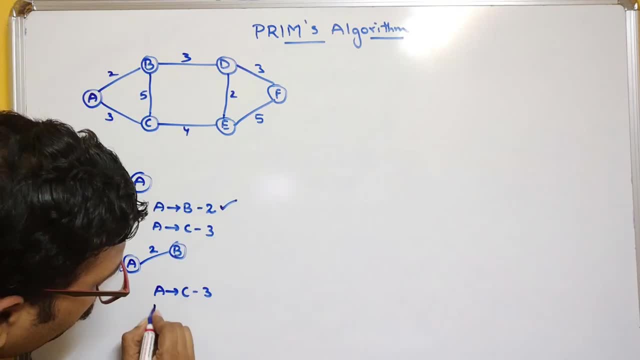 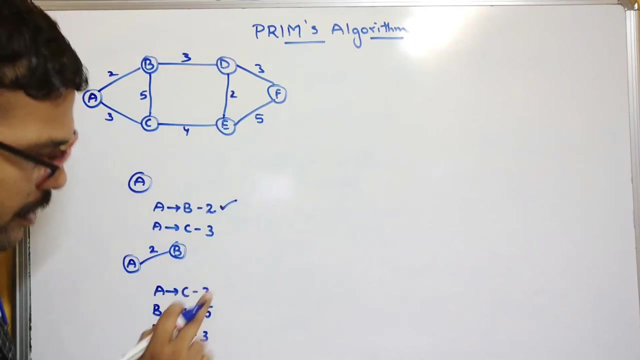 So we need to consider B to C and B to D. So B to C with a cost of 5 and B to D, B to D with a cost of 3, right, B to A, B to C, B to D. right. Now, what happens Among this? 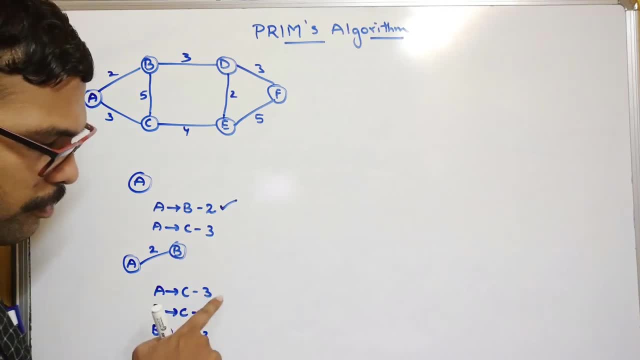 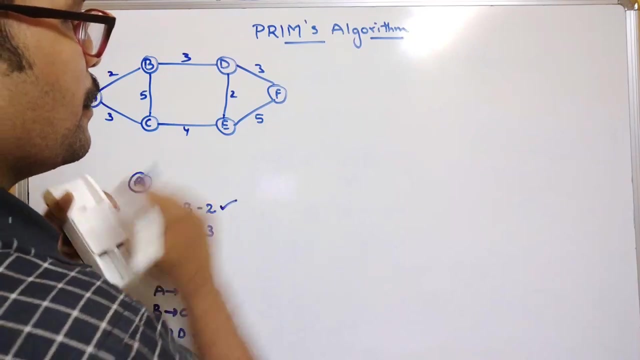 one. we are having two edges with a minimum cost of 3.. So you can select any edge, no problem. So I will select this one B to D. I will select this one B to D Now. the tree will be A. The tree will be A followed. 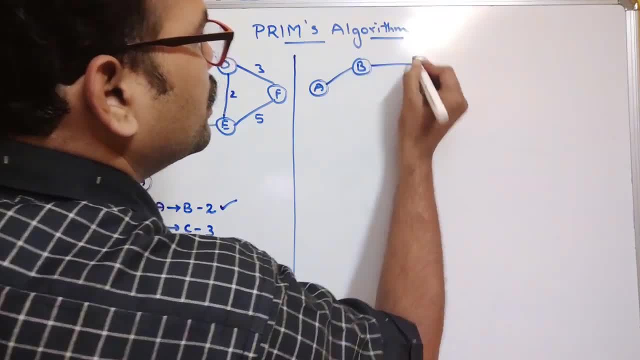 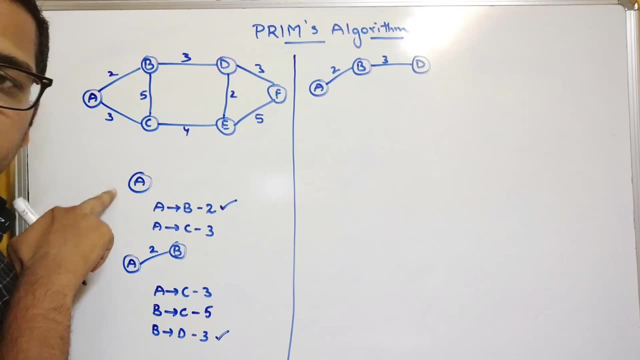 by B, B to D, So the edges are 2, 3.. Now the spanning tree becomes this one. So in the first step, that the spanning tree is this one, that means only one vertex. In the second step. so, first step, this one. 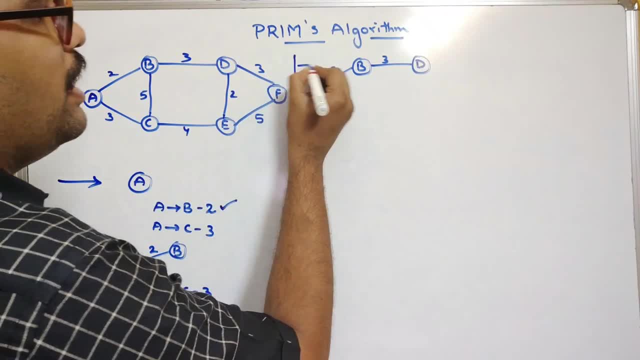 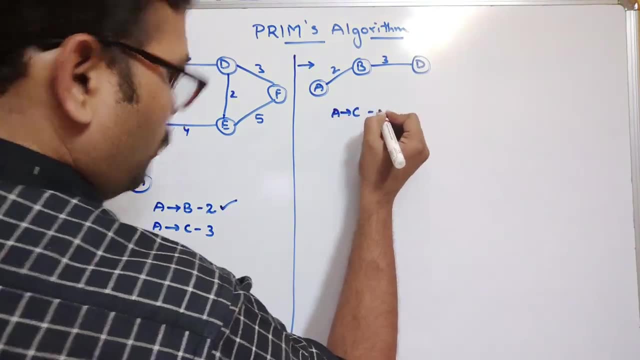 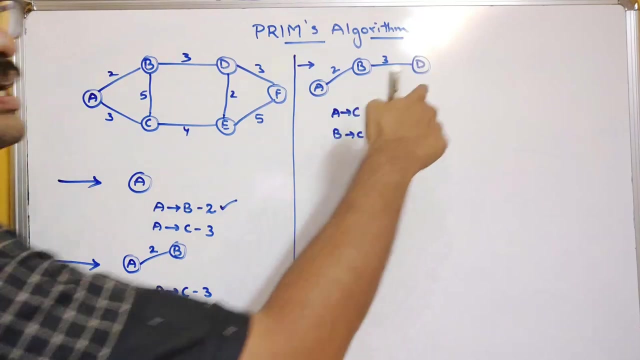 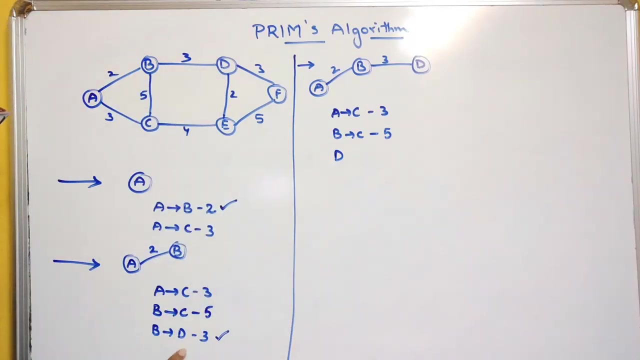 Okay, Okay, second step, and this one is the third step. now consider the remaining edges. what are the remaining edges? a to c with a cost of 3, b to c with a cost of 5. right now, d is added here. now consider the edges of d so you can see d to b, which is already done because of undirected right. 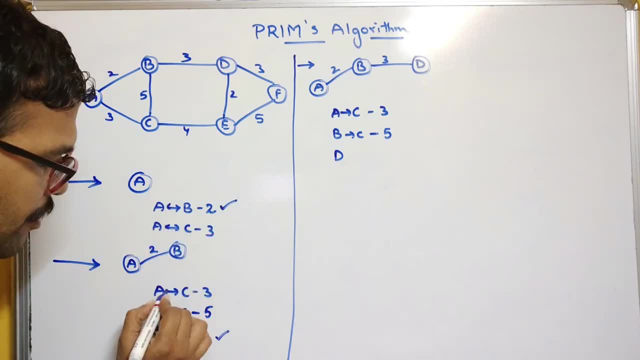 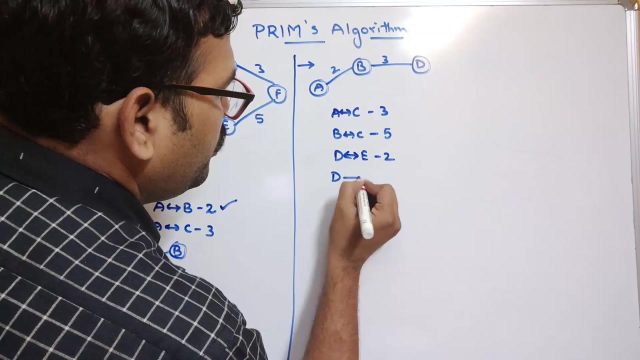 so you can simply use this one bidirectional right right. so b to d is completed now b to d to e. so d to e with a cost of 2 and d to f with a cost of 3 right. so all the edges of d are d to b. 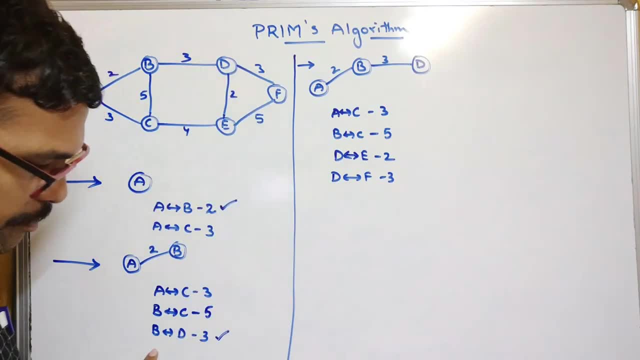 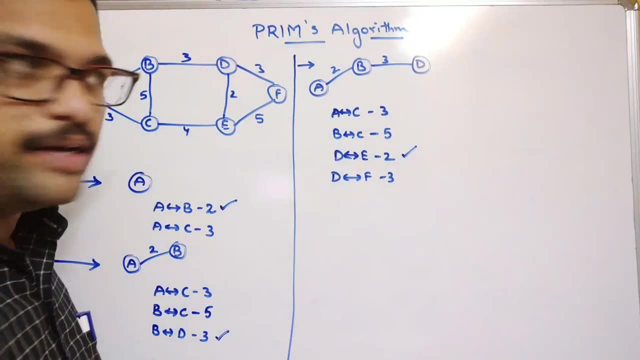 d to e and d to f. so among the d to b is completed right now. among the edges of d to b is completed right. so among the edges of d to e is completed right from these. what is the minimum cost? so this one, least edge, least weighted edge. so consider this: 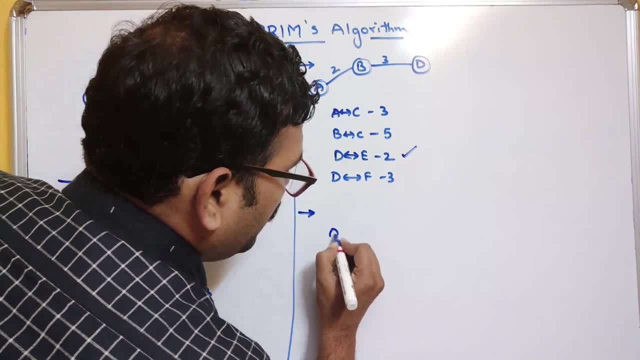 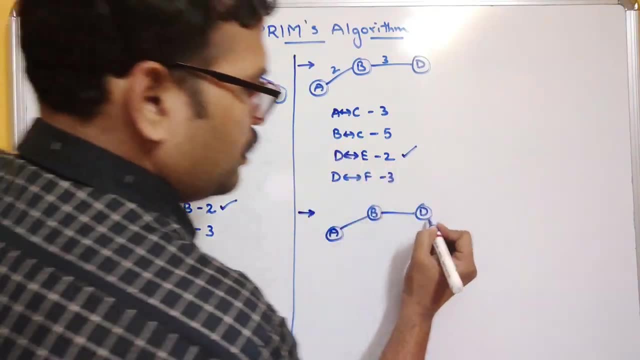 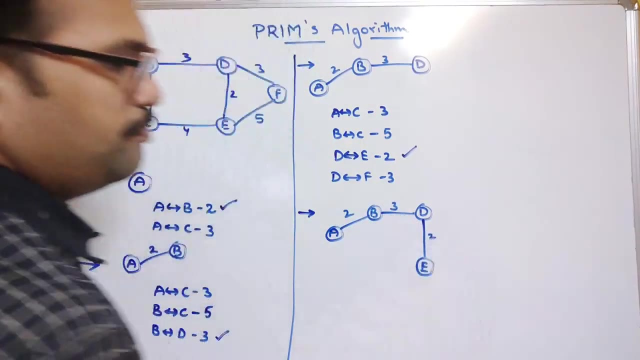 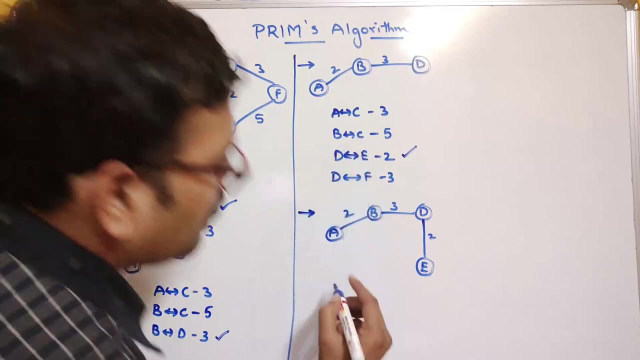 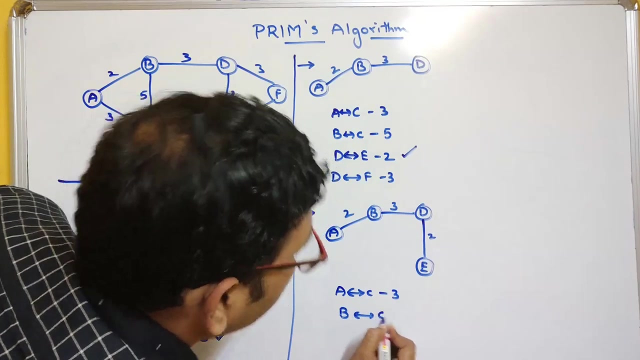 one. now the spanning tree will be a edge to b, edge to b and from d to e, e. so the cost is 2, 3 and 2. cost is 2, 3 and 2. right, and next next correct. what are the remaining edges? simply right here: a to c with a cost of 3, b to c with a cost of 5. 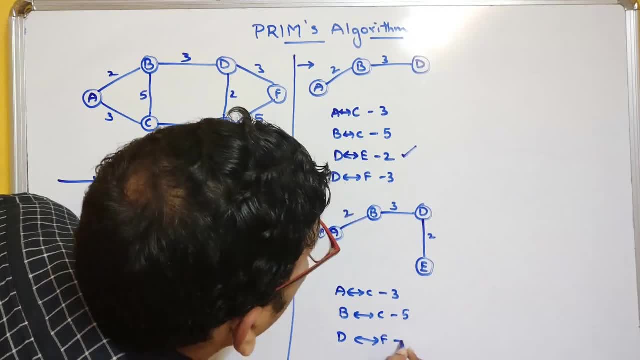 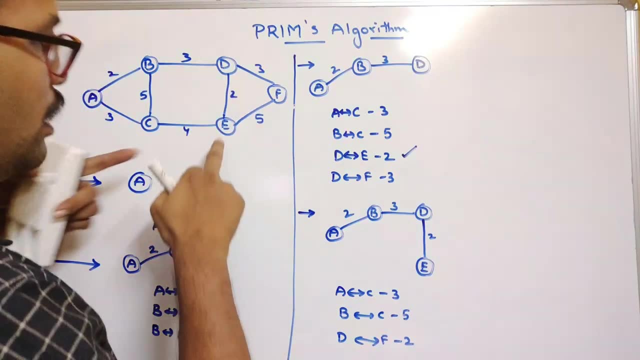 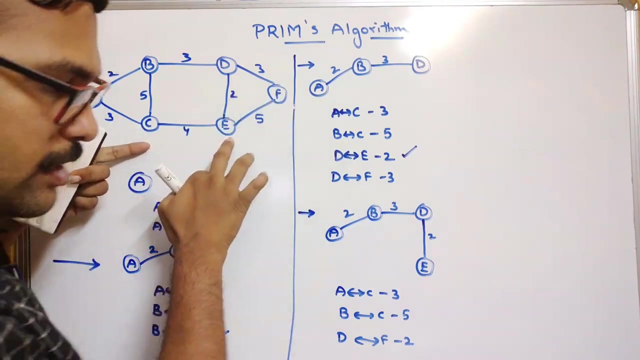 and d to f with a cost of 2. now e is added. so what are the edges of e? e to d, e to c, e to f. so e to d is completed. now just discard that one, e to c. so e to c is not there, so we can write the. 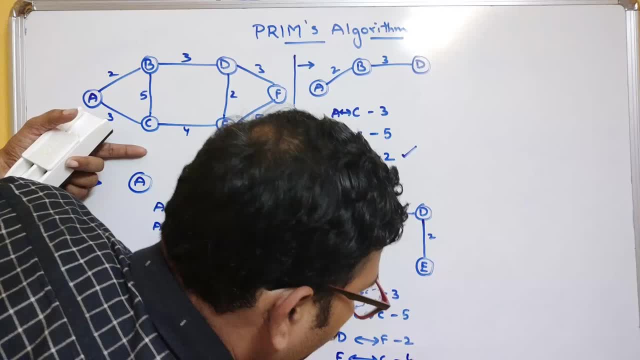 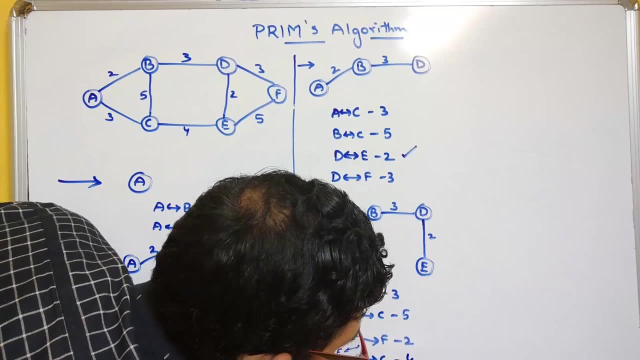 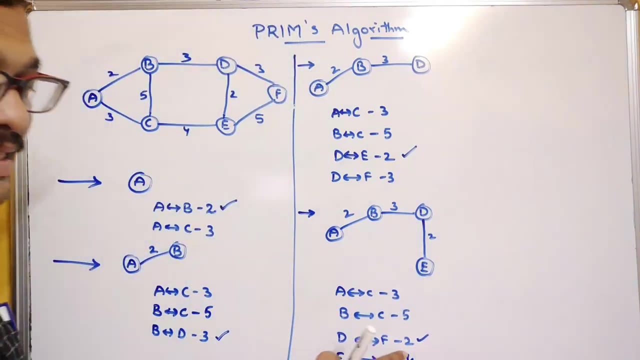 edge: e to c with a cost of 4, and e to f with a cost of 5. e to f with a cost of 5. e to f. right now, among this one, this one is the least weighted edge. least weighted edge: d to f. so 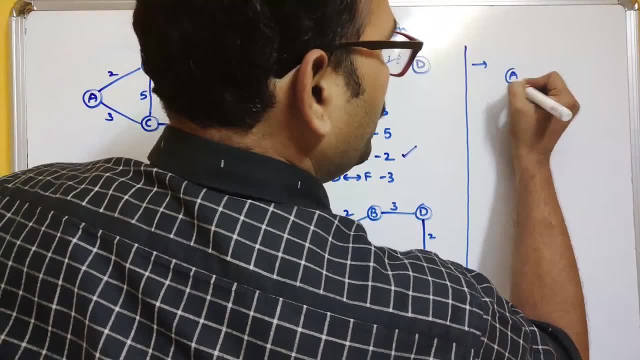 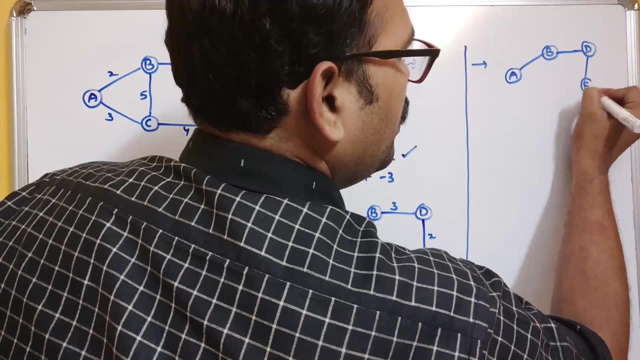 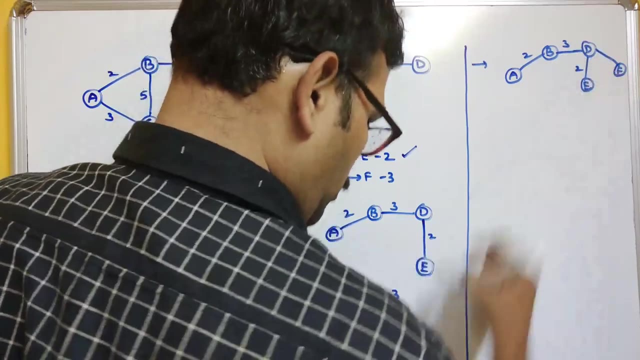 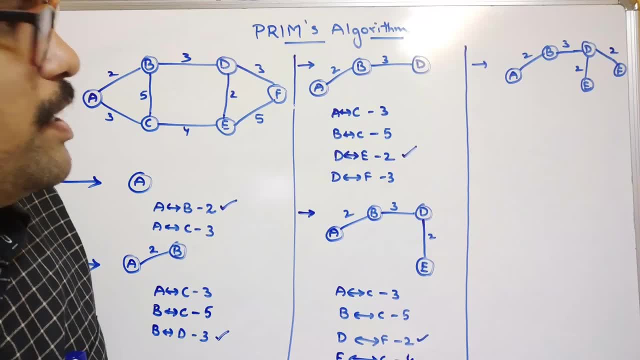 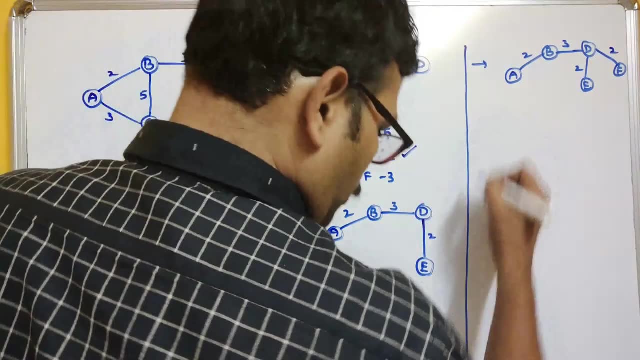 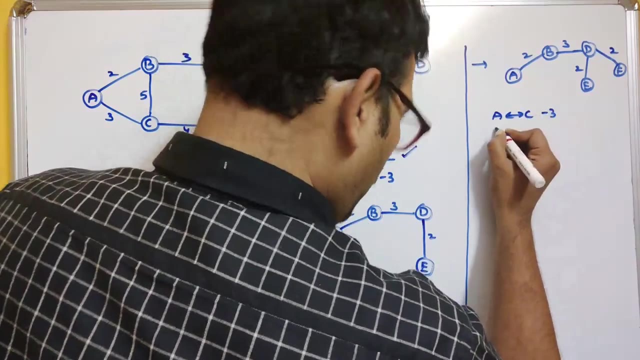 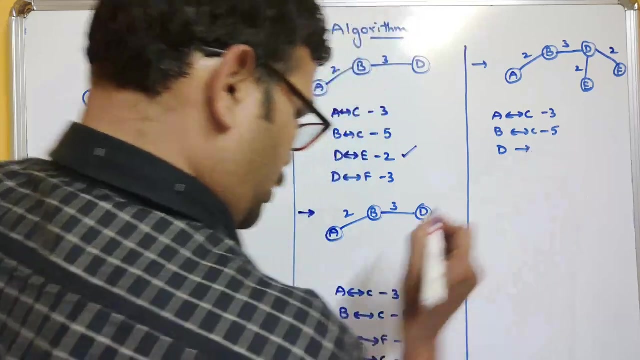 whether all the vertices have been covered or not. a, b, b, so there is no. C is not there, right? so you can continue the process. So what are the remaining edges? A to C, with a cost 3, B to C with a cost 5, E to C. D to F is completed. 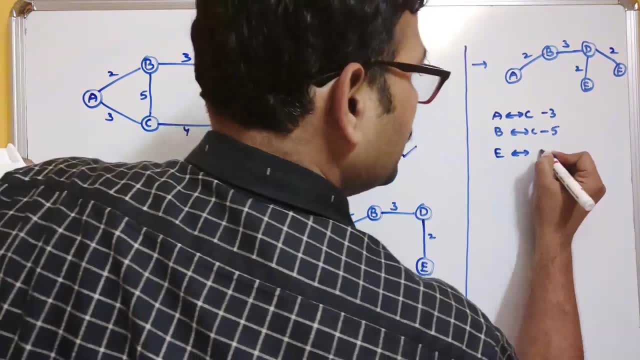 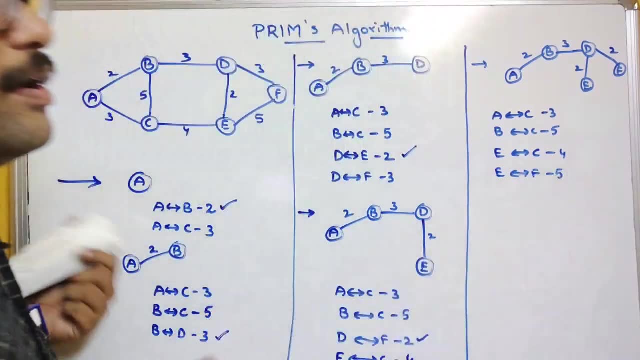 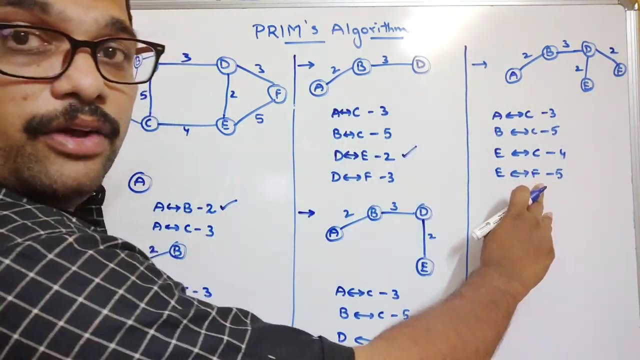 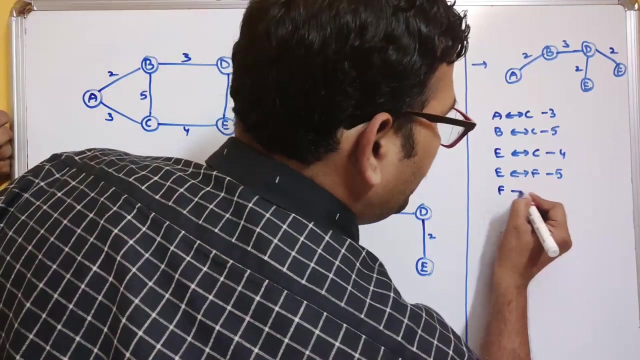 So E to C with a 4, E to F with a 5, right Next F. we have reached to F. So the new vertex is F. So write down the vertices of F. So F to D, F to E right F to E is completed. So F to D with a cost of 3.. 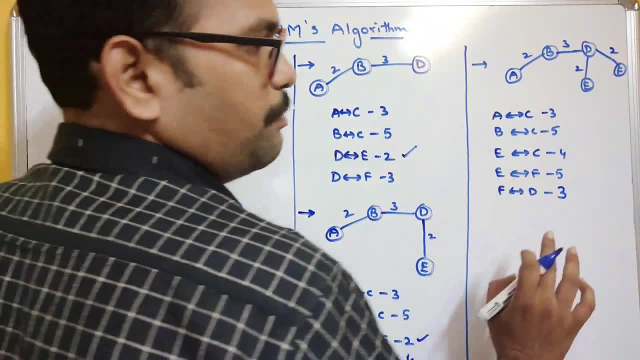 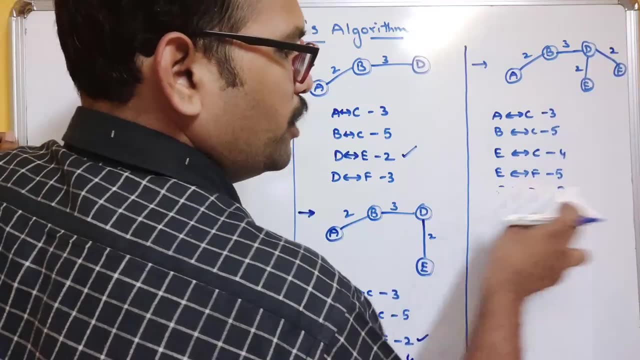 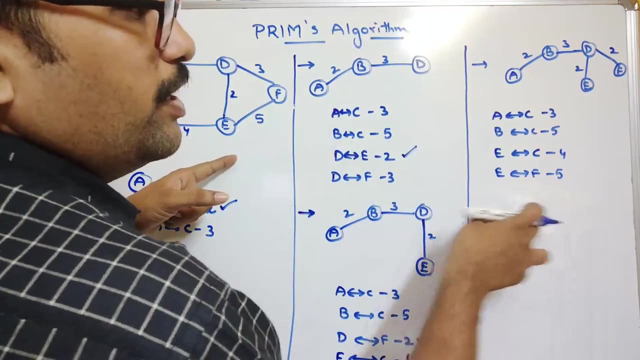 Now you can see among all these things what is the minimum: A to C or F to D. right F to D is also completed. right F to D is also completed, So you need not go with this one. And one more thing is F to E, So that is also completed. F to E. We have written F to E here, right? 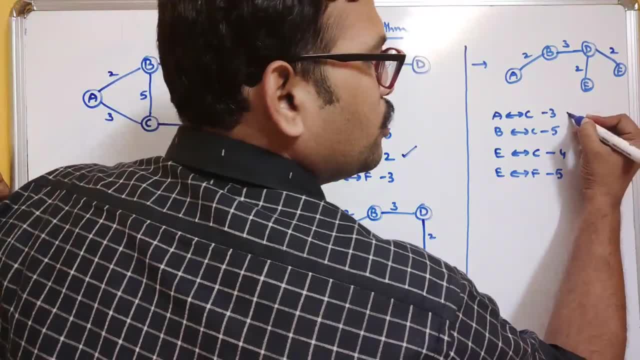 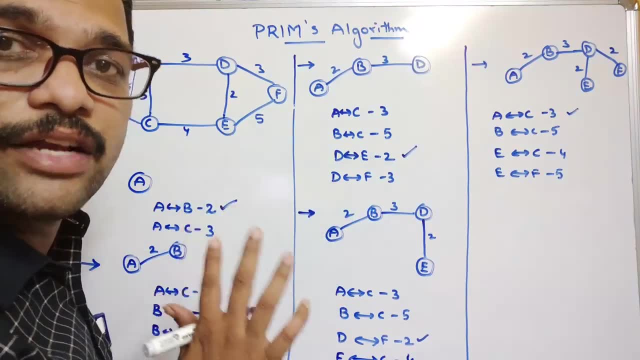 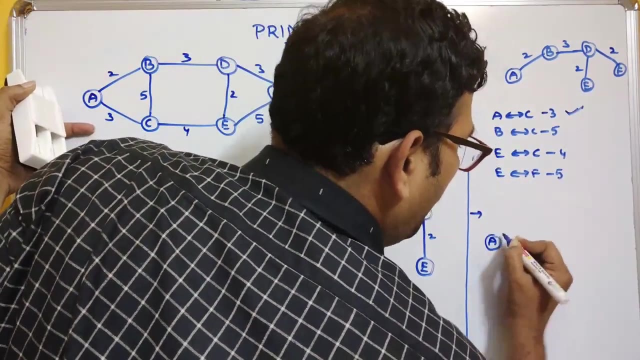 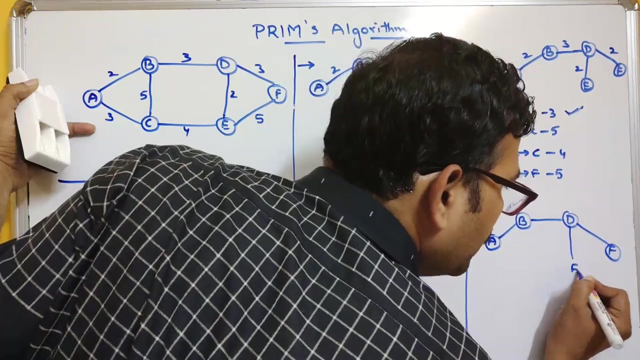 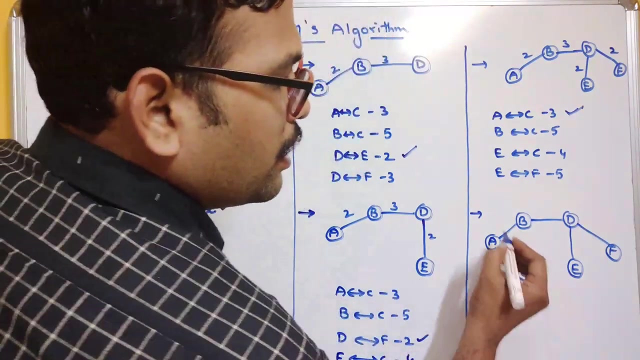 So now, among all these things, what is the minimum cost? A to C. So consider A to C and observe whether it is giving the cycle or not. It forms a cycle or not. So if you, If you, apply A to C, it does not form the cycle. So consider this one. So A to B, D, F, E, C, right Now you can give the weightage 2, 3, 2, 2 and 3.. 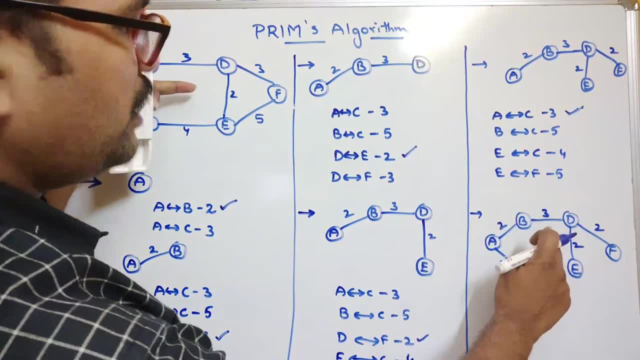 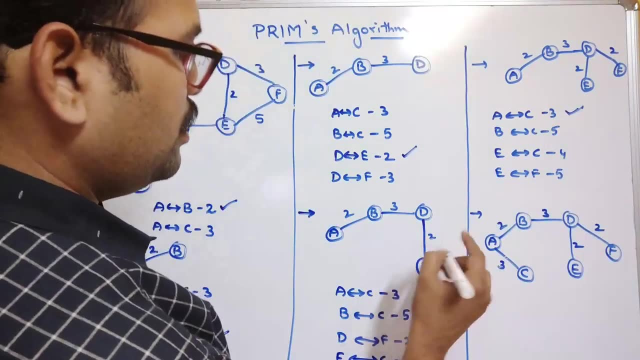 So you can observe here: A to B with 2, B to D with 3., D to F with 3.. D to F with 3.. So D to F, 3.. Okay, D to F is 3.. 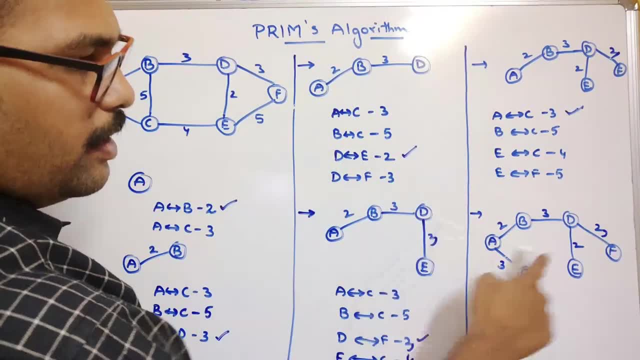 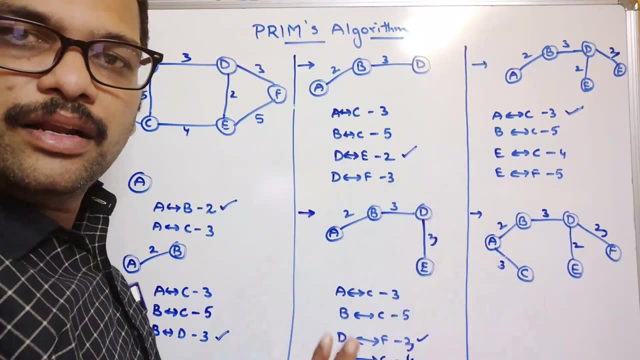 So this is D to F with 3.. And then D to E with 2, and A to C is 3.. So you can observe, here all the vertices have been constructed. That means included in the tree. So A, B, C, D, E, F. 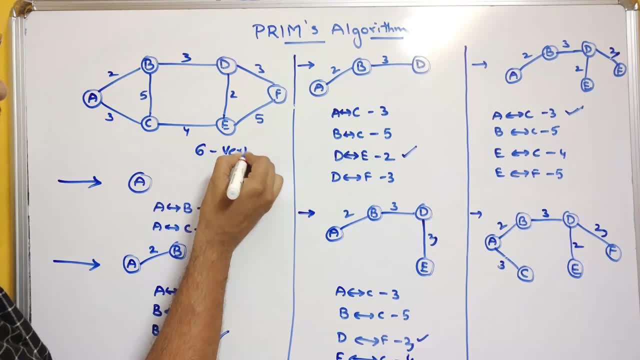 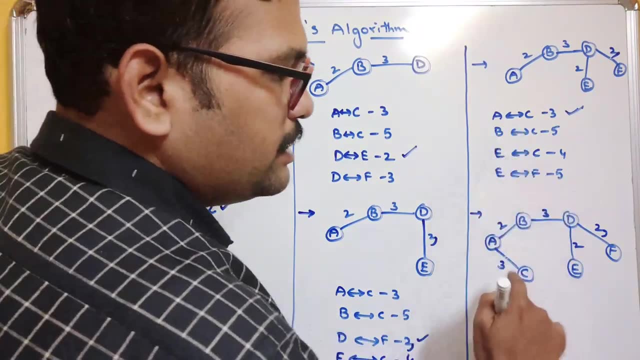 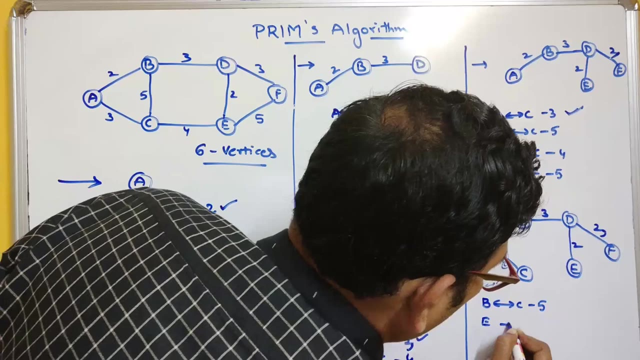 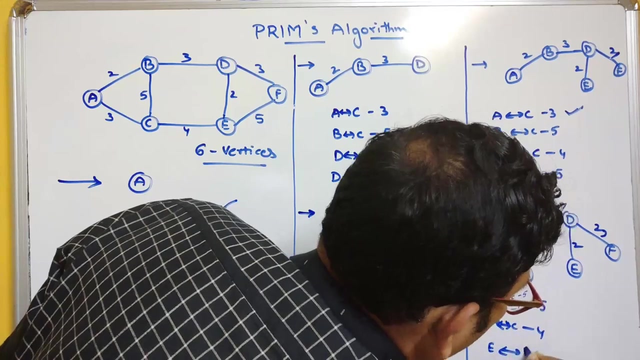 So here we are having total 6 vertices, 6 vertices. So all the 6 vertices have been included. And now you can observe here the remaining edges. What are the remaining edges? So consider B to C with a 5 and E to C with 4 and E to F with a 5.. 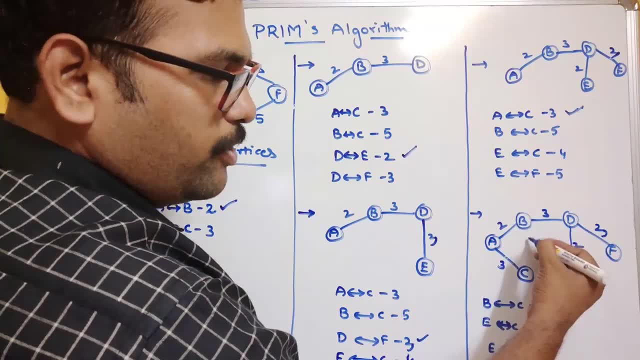 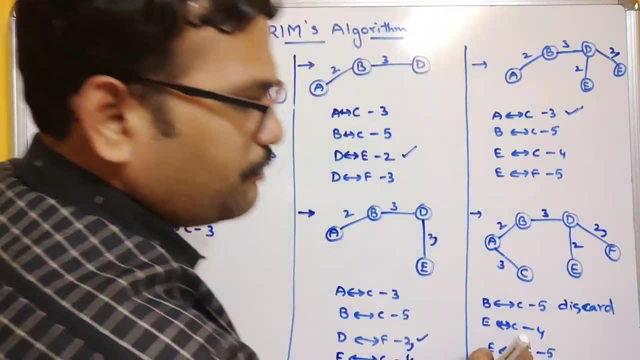 So if you consider B to C, So if you add a B to C, it forms a cycle. So we have to discard this one Right. E to C: 4. E to C: If you just connect this edge again there is a cycle. 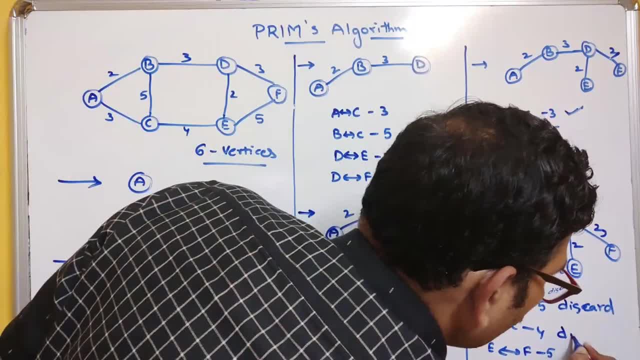 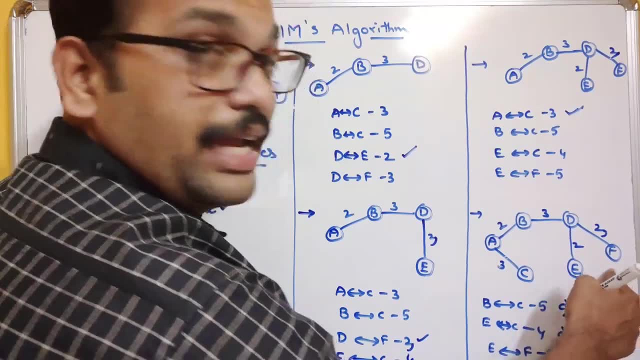 So A, B, D, E, C, A. So again you need to discard this edge And E to F Again. if you connect this edge, E to F, again a cycle forms. So again we need to discard these edges. 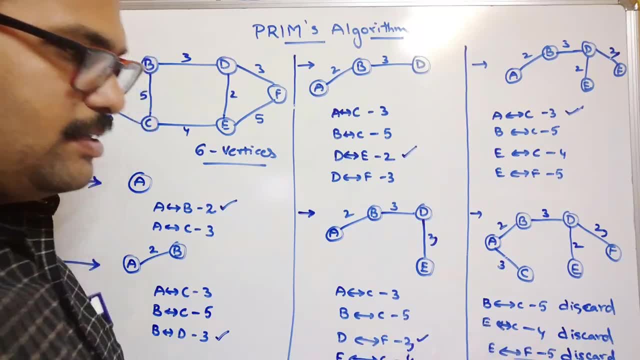 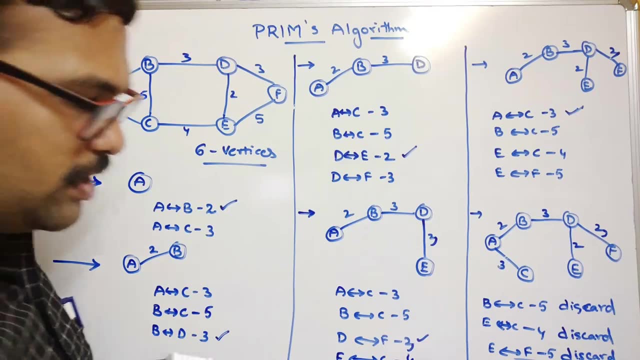 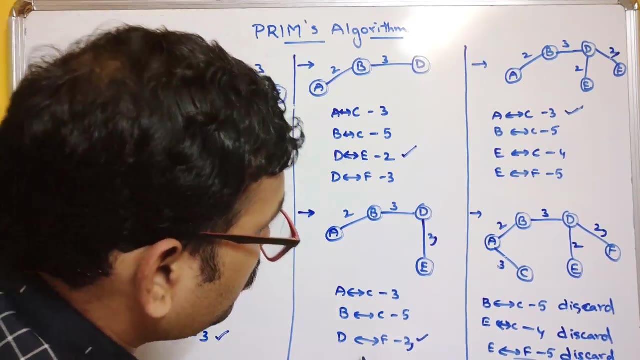 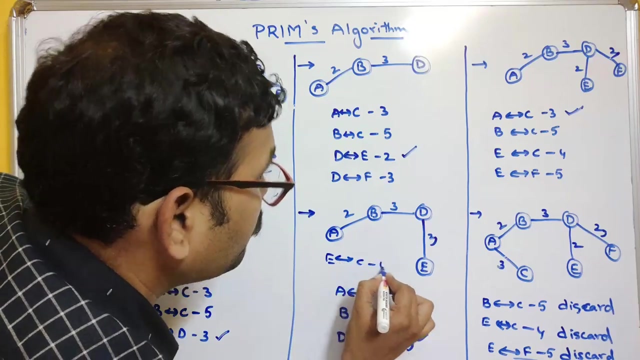 So we have to discard These edges so that we can have this one. Okay, So hope you got this one. So I think these things are not clear, So I will write the edges here: E to C with a 4 and E to F with a 5.. 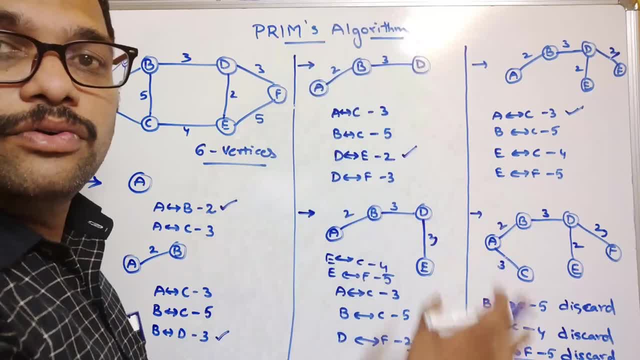 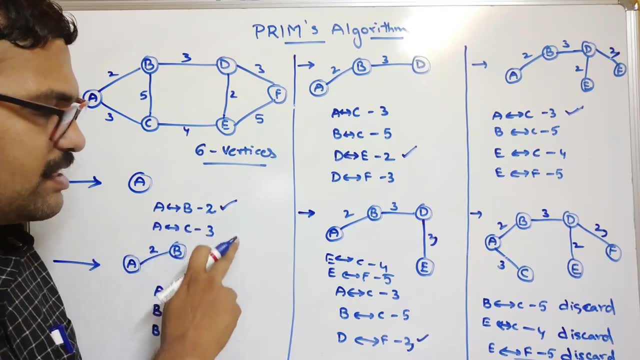 Right. So I think now it's clear. So we have to apply, We have to consider: from this single vertex You can consider any vertex And consider the edges, All the edges from that vertex to new vertices, And consider the least weighted edge. 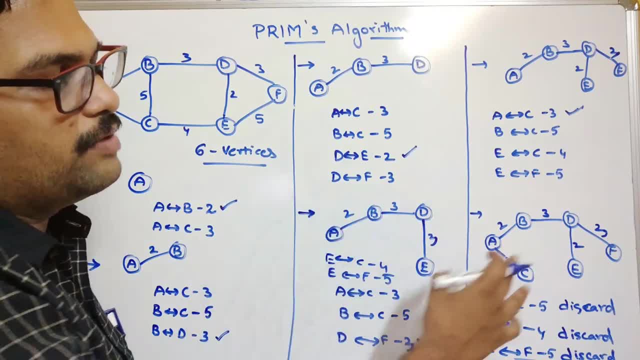 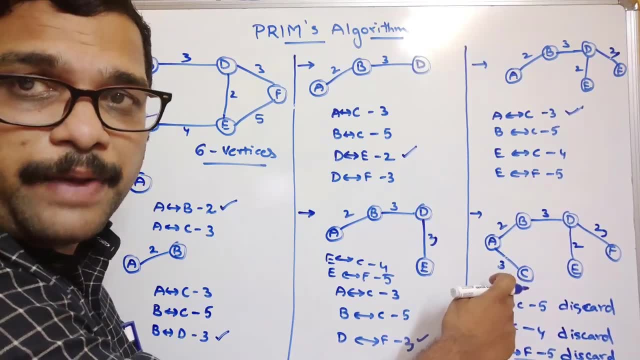 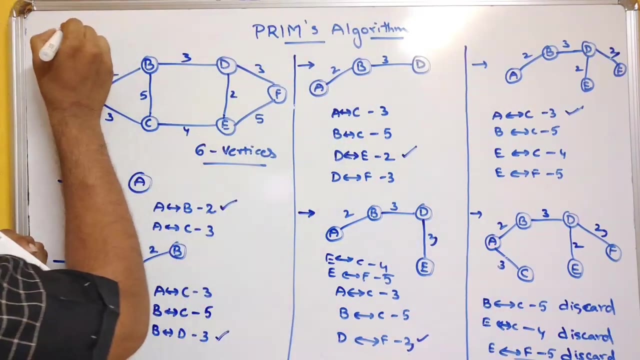 Okay, And continue the process until all the vertices will be connected. So this is the spanning tree. Minimum cost spanning tree. Minimum cost spanning tree for the given graph. What is the cost here? So you can observe the cost, I will write here. 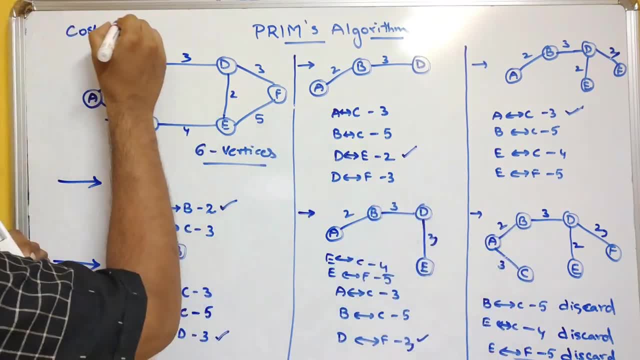 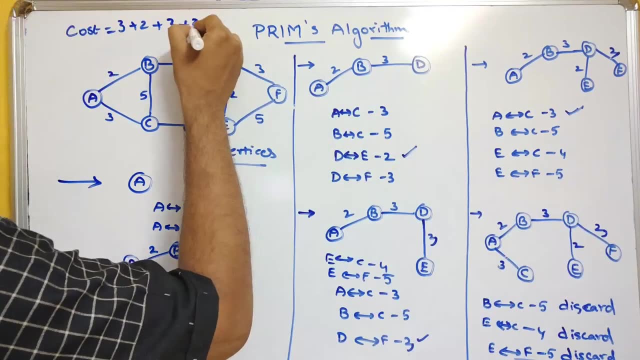 Cost is equal to. So what is the cost? 3 plus 2 plus 3 plus 3 plus 2.. 3, 2,, 3, 3, 2.. So what is the total cost here? 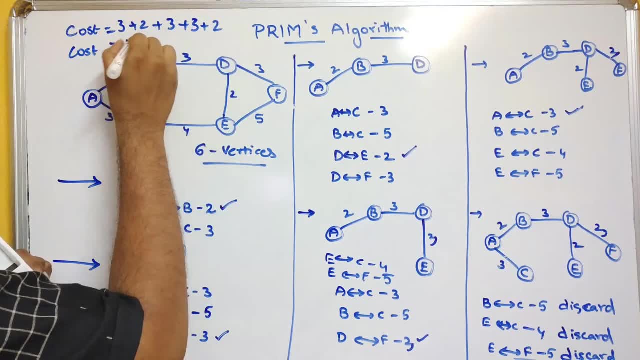 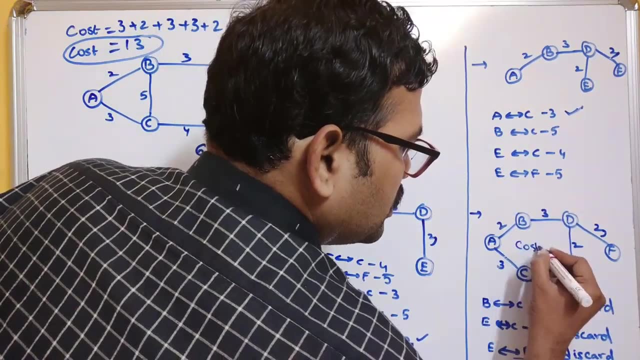 You can observe, So 5,, 8,, 10,, 13.. So 13 is the minimum cost for this particular tree. So 13 is the minimum cost for this particular tree. So the cost, The cost is 13.. 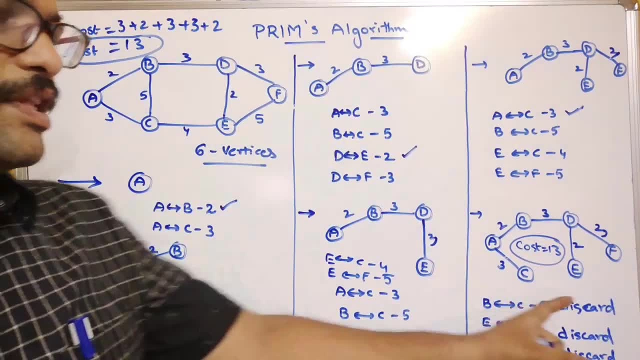 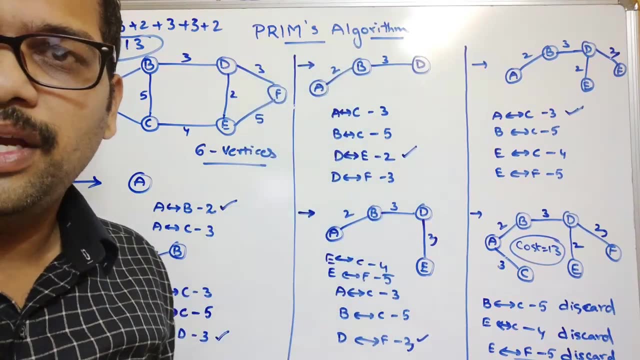 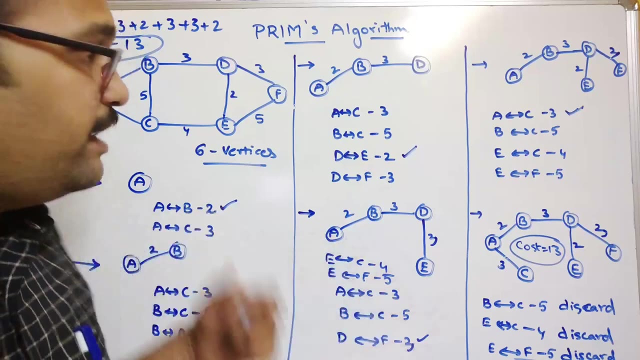 The cost is 13 to construct this particular spanning tree. So this is the procedure we need to follow for Prim's algorithm. Okay, So consider a graph And finally, we are getting the minimum cost spanning tree. So we will get many spanning trees from this graph. 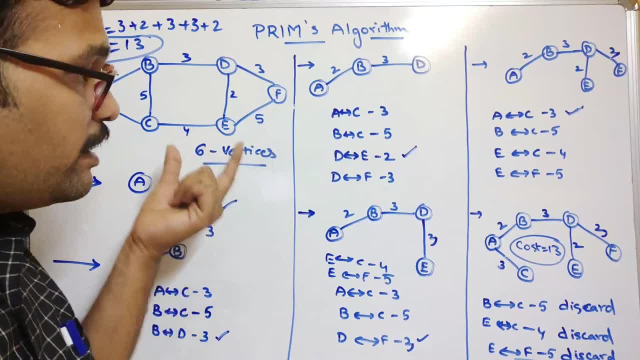 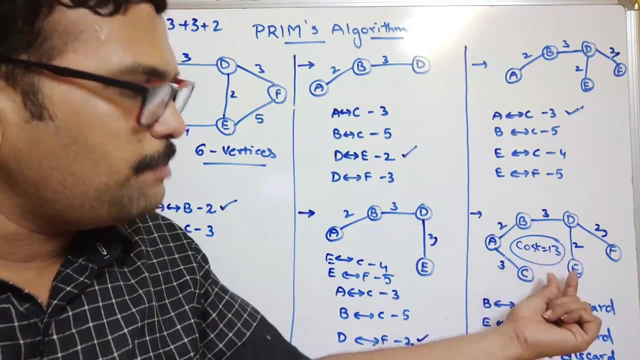 So, as we discussed in the previous session, Right, So we can get many spanning trees from this graph, But, But we need to find out the minimum cost spanning tree. So this is the minimum cost spanning tree obtained from this particular graph. 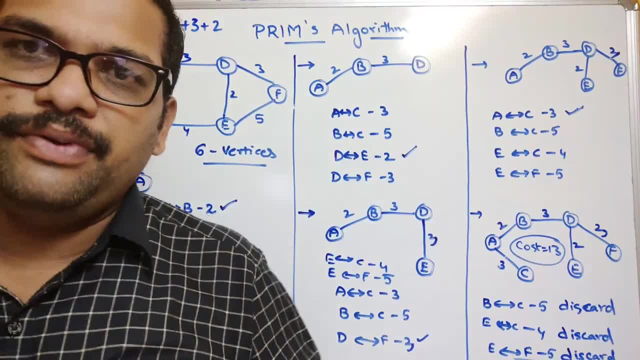 So hope you understood this one. So if you are having any doubts regarding this one, Feel free to post your doubts in the comment section. Definitely, I will try to clarify all your doubts And if you really enjoyed my session, Like my session. 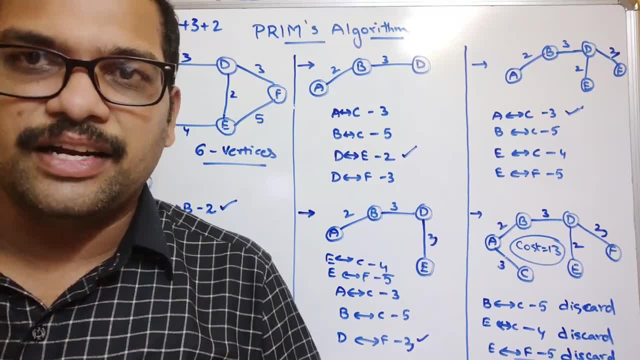 Share my session with your friends And don't forget to subscribe to our channel. Thanks for watching. Thank you very much.